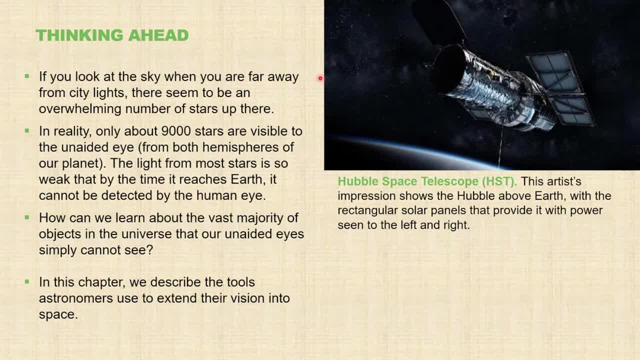 Even without the light pollution. But we know now that there are millions, billions of stars within the Milky Way galaxy. So how can we detect or observe those stars With? you know, without or our, that our unaided eyes simply cannot detect. 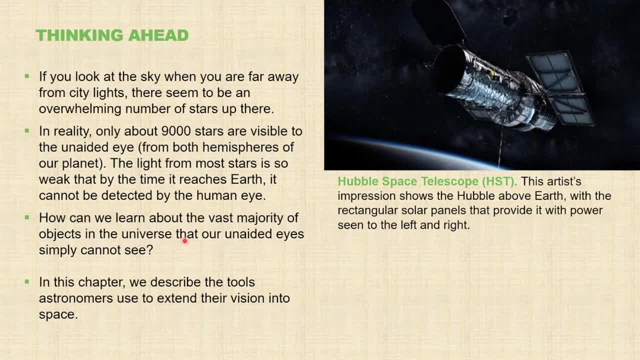 Simply cannot see. And here is an example of a space-based telescope. You all have heard of the mighty Hubble Space Telescope. It was the most powerful space-based telescope since it was launched, And it is still. However, the story is changing. 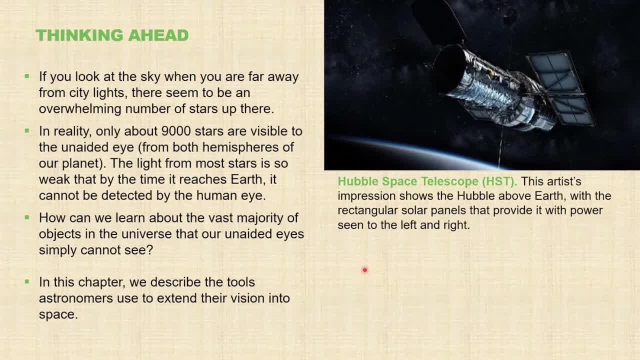 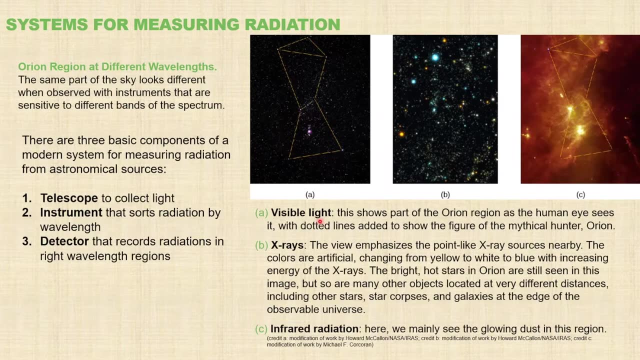 The history is being rewritten. You may have heard of James Webb Space Telescope That we will look into today. briefly, Okay, there are three basic components of a modern system of measuring radiation. We call it radiation because, now you know, radiation consists of the whole spectrum. 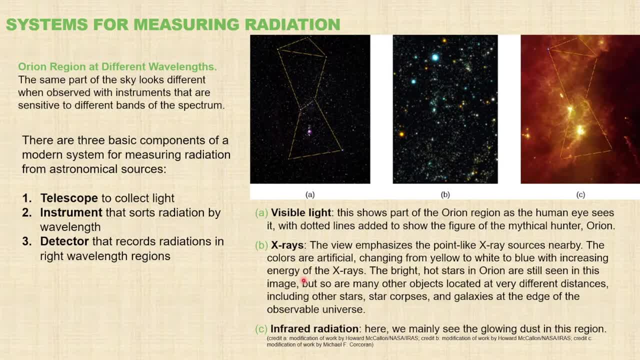 Ration is a function of the wavelength of light extending from gamma rays to radio. Here you see the wavelength of light extending from gamma rays to radio. In the visible portion that we see, we use optical telescope Like this one here. This is based on the visible light. 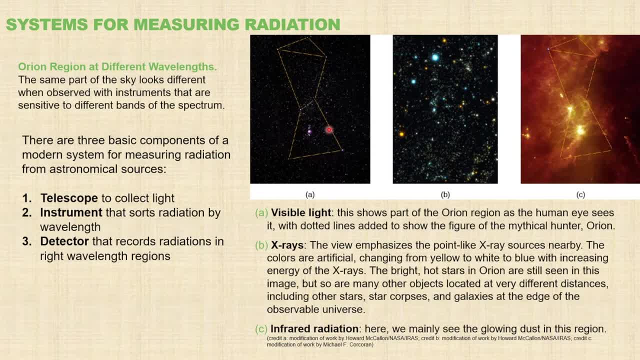 We're looking at Orion region, Orion constellation, And this is the Orion's belt, And this is the Orion's belt by using a visible telescope or you know, the this part of the sky. this constellation looks like this and and be here. this is the same reason now looked. 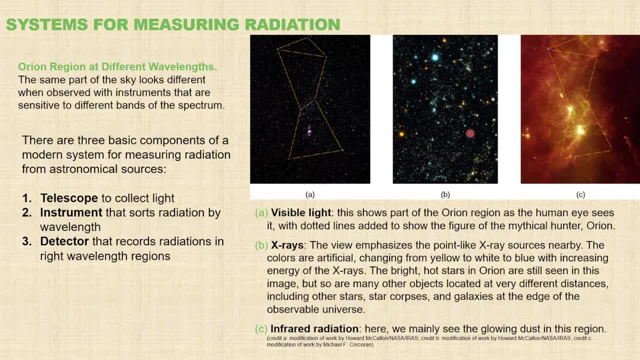 by a different lens and now that lens records the x-ray coming out. from that reason x-rays not visible light, but x-rays little stronger part in our spectrum and this one here on. the third one is the infrared. infrared radiation. when things get hot, hotter object emit infrared radiation like, right, our body. 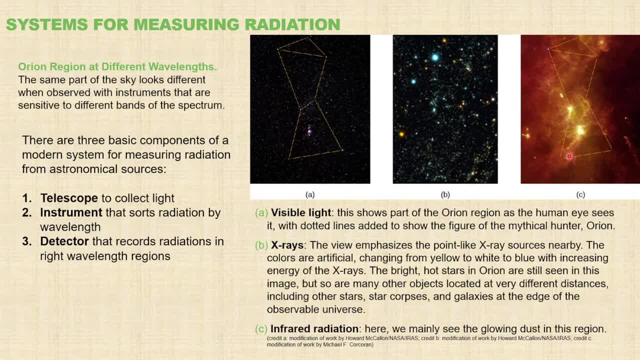 right now. if my eyes could detect infrared, infrared radiation, you'd all be glowing like this one here: the, the gases around. this reason here observes the, the radiation from the stars, from galaxies, and they emit that infrared. and the infrared camera in the infrared telescope detects this reason in this. 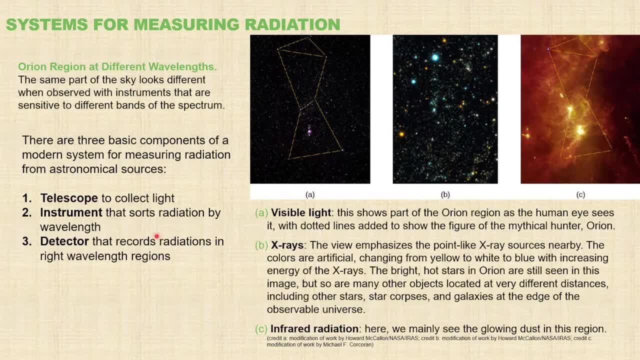 color and again the basic components: telescope. they collect light. simply it's like a bucket gathering water. they collect light, they collect photon and that photon are directed now into instruments where those instrument can short different wavelengths of that light collected, wavelengths of those photons collected. and now those photons are. 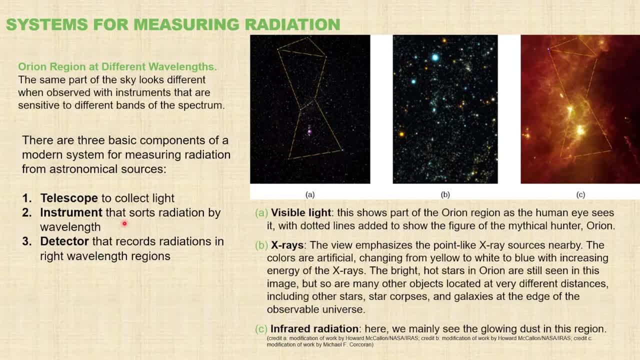 directed into certain part of the detector, within the telescope or away from the telescope, and those detectors detect those radiation at different wavelengths, like this picture here, can you know, be taken with one telescope, and the x-rays can be detected. sorry, directed to one detector, where it puts. 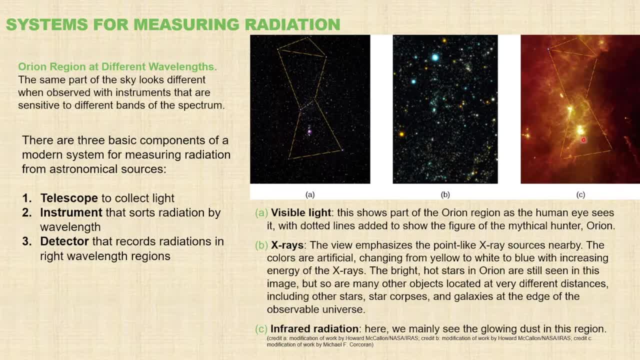 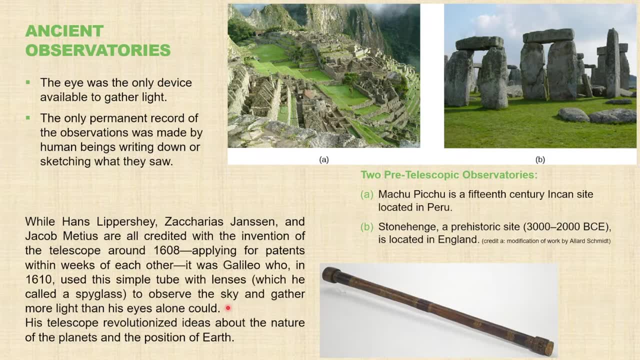 out this image and the infrared waves can be directed to another device which puts out this image here. but even you start this way, of course. look at the first telescope built by Galileo to observe the, the planets, the Wanderers. what are you called? Mercury, Venus, Mars, Jupiter, Saturn, even. 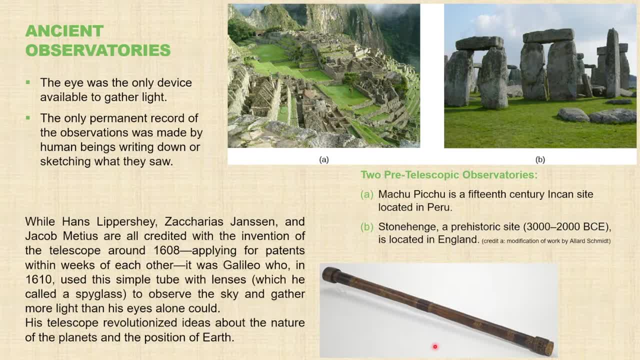 เส pins the moons of Jupiter using this simple device in 1610.. However, this device was- I mean Galileo used it in astronomy extensively. There are other claims from these inventors: Hans, Zacharias, Jacob. they filed for the copyright as well- credited to the invention. 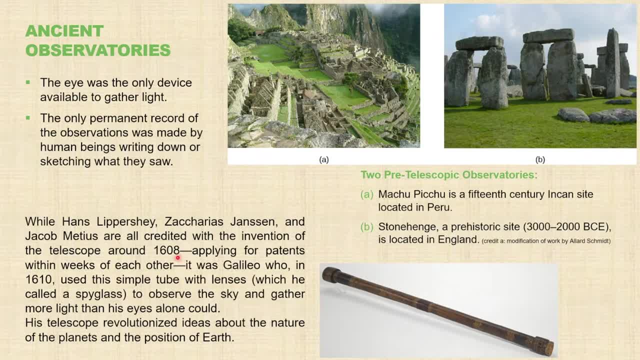 of this telescope around 1608.. They have patents to it, So maybe you should not give entire credit to Galileo, but Galileo definitely used it for the astronomical purpose And the before telescope. there were observations made and we still do it today And we see something. 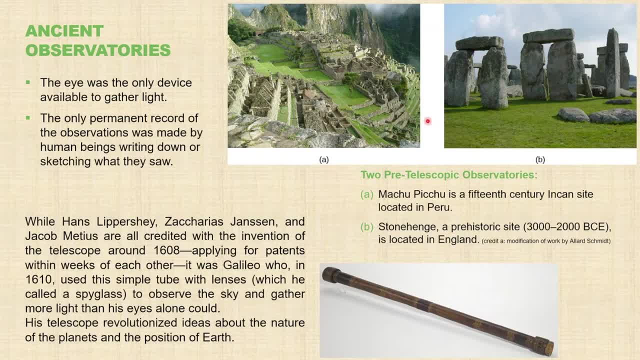 we write down and for that purpose, certain places were built, like this, Machu Picchu and the Stonehenge, But this was all based on what you see, whatever eyes could gather and whatever you see, then you had to write it down, log it in a book Or creative people. 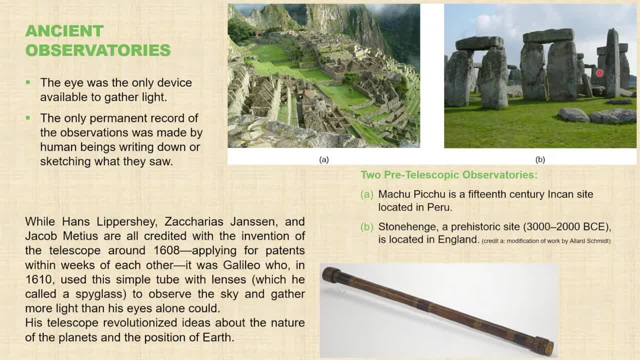 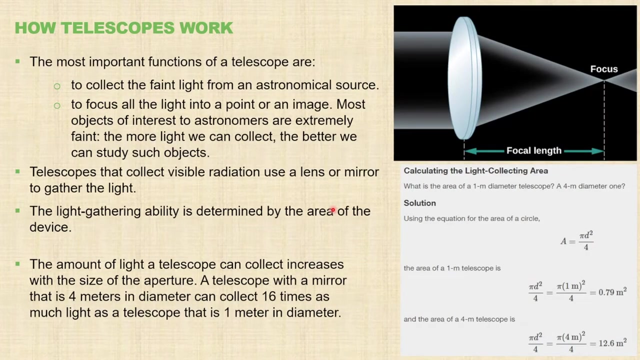 sometimes they draw and keep that as a record. And this telescope here- a wooden piece, maybe a bamboo, you know- had some lenses inside, later evolved into some of the biggest telescope. So how does telescope work? Simple, it collects from the astronomical sources. could be stars, galaxies, nebulas. 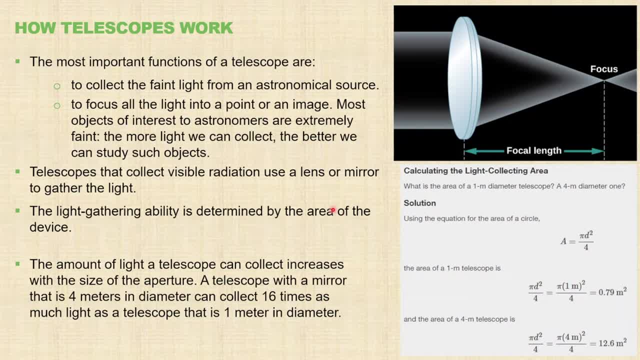 and, as such, And all of those light are focused into a certain point. where now we place a detector, we detector collects all that light and forms a ha Gog pregunt – 1 Th Ra and 1 Th Z. And you see, the first telescope was pretty thin, So the area of 2端 thinner than the greater. 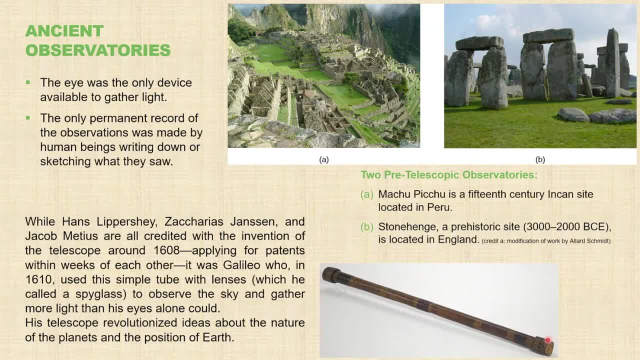 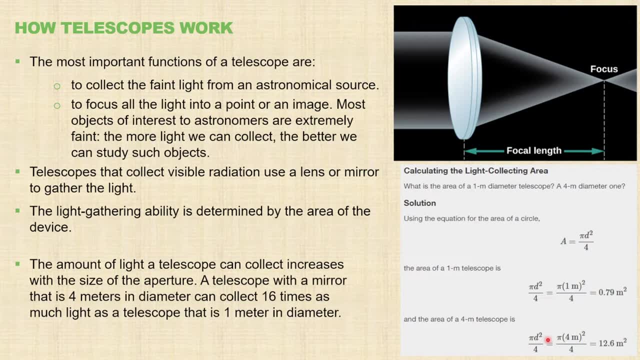 area of the lens was thin, small. Later we realized if we can increase the size of the area, more light can be collected from a fainter star. We only see brightest stars, Yet stars that are much farther out, the galaxies that are much farther out. 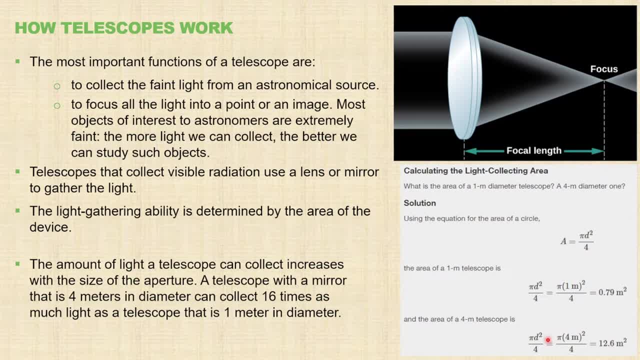 they give out very faint light that we cannot see. But if you have large enough area and increase the exposure time, meaning collect the light not for a few millisecond or a second- that our camera does. you know these telescope, they open up for hours, days. 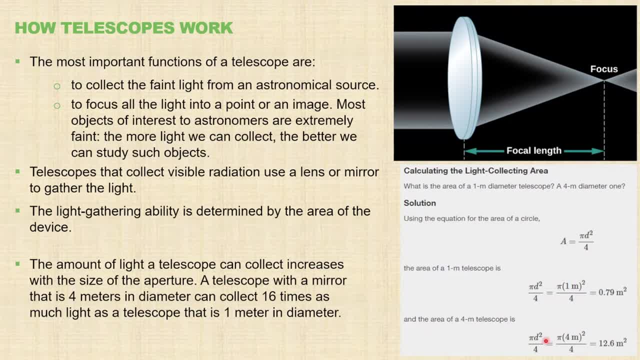 basically collecting the light coming in and produce better, high resolution, crisp images. And again, larger area means more light can be collected. For example here: if a lens has one meter diameter versus four meters diameter, the calculating the total light collecting area, 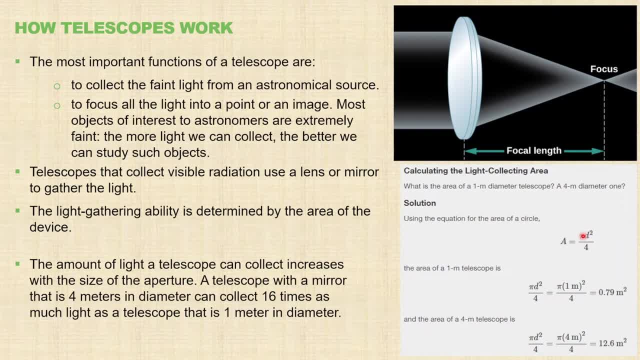 it's simple area is by R square pi times. radius is square, but radius is after diameter. Put in that formula, for one meter telescope has 0.79 meters square. four meter telescope gives 12.6 meters square. That's a factor of 16 difference. 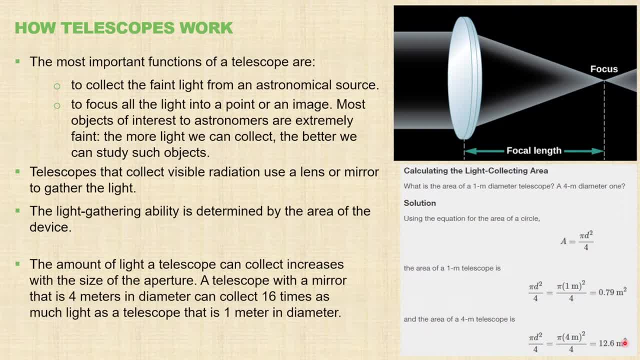 So having one meter diameter telescope compared to 16 meter diameter- sorry, four meter diameter telescope, one meter diameter telescope can have the can collect 16 times more light, hence produce better image. high resolution image, high quality image. Lens have certain properties. 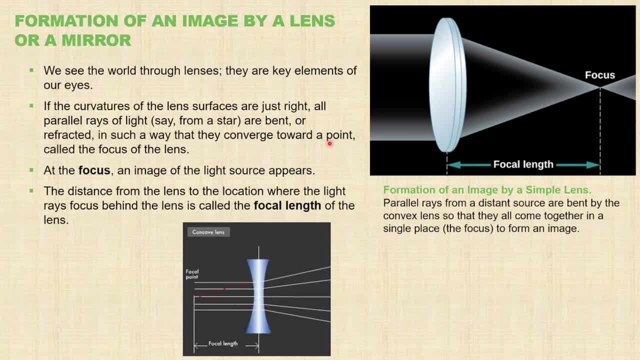 and there are different types of lens. Two mostly widely used are the convex lens and the concave lens. Convex lens have these: this is concave See, this is convex, the bulging edges. So when light, the parallel light, 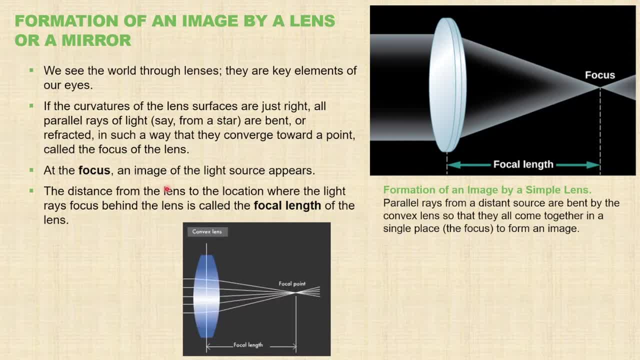 usually the light coming from distant source- sun or other stars- are parallel by the time they reach here, due to the distance they travel. This parallel light rays are converged by a converging lens or convex lens to a point called a focus or a focal point focus. 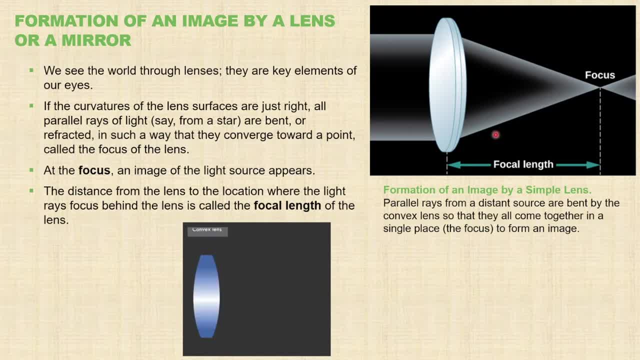 So the light rays here coming from distant source, they're converged. So image is formed at the focus by a convex lens. The other lens is diverging lens. It diverges the light rays, but we can have a diverging mirror instead. 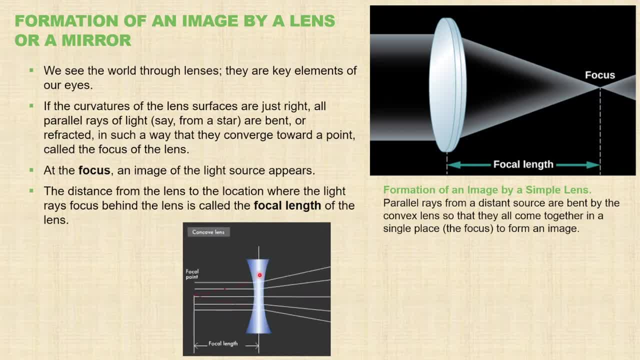 So if we polish one side of this diverging mirror here, polish it on this side so it reflects back to again its focal point where the image is formed. So we can have a converging lens telescope or we can have a telescope that have mirrors in it. 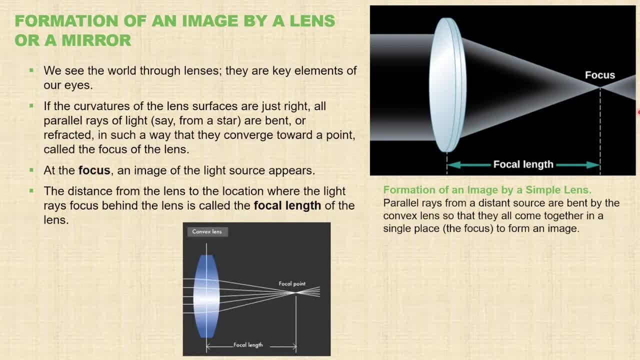 But again, these are some of the technical terms. The focus is where the parallel light rays are converged And this depends on the size of the lens, thickness of the lens. This means the length, distance to the focus, which is called the focal length from the lens to the focus. 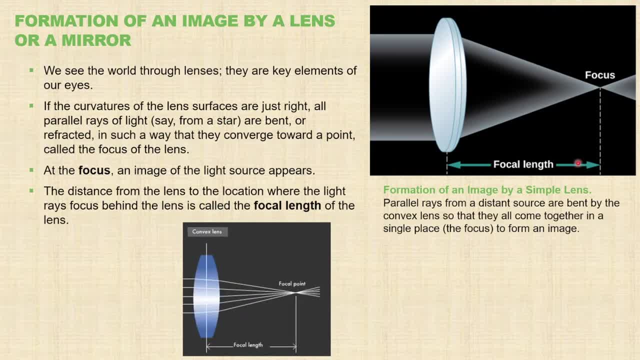 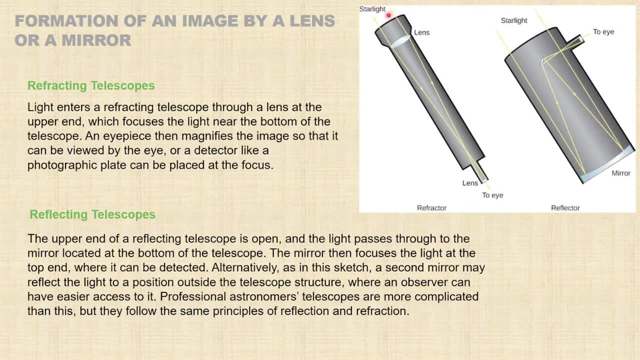 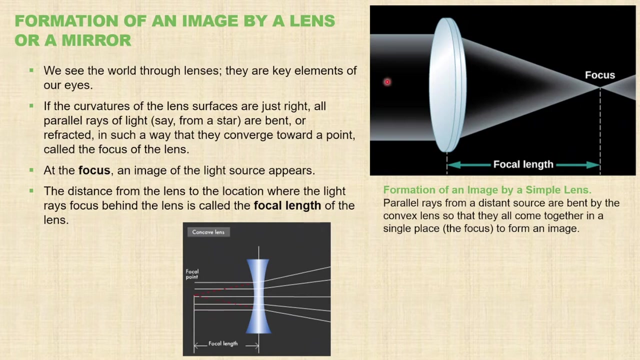 This is called focal length. This length can decrease or increase depending on the size of the lens itself. And so now, basically, for inside the telescope. here the starlight enters the opening of the telescope. Like this is the starlight. here The ray model is given down. here 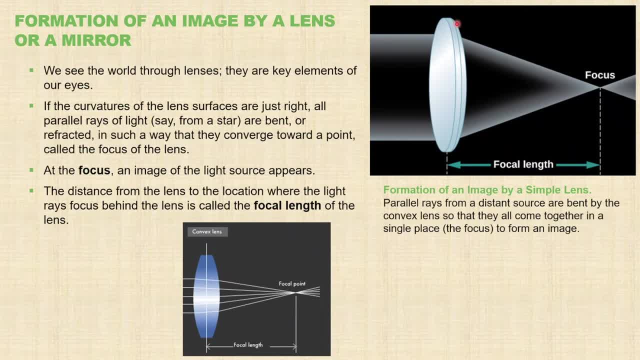 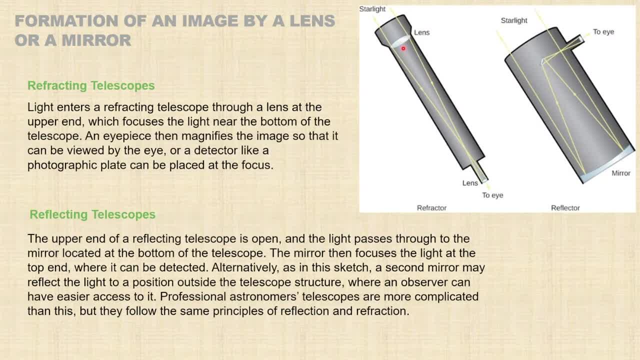 which converges the light to a single point, which is a little bit like a green dot across plastic. Then the focus: here this lens has a focal point around that region here. Then the focus: here this lens has a focal point around that region here. 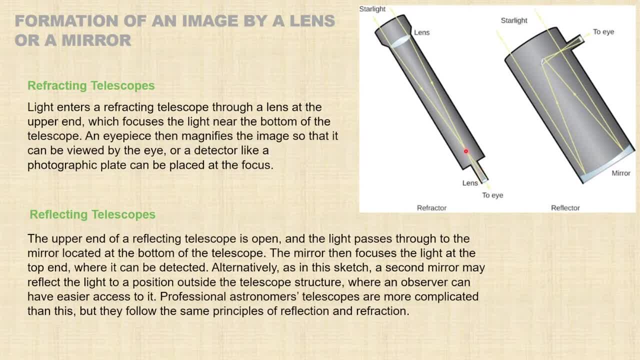 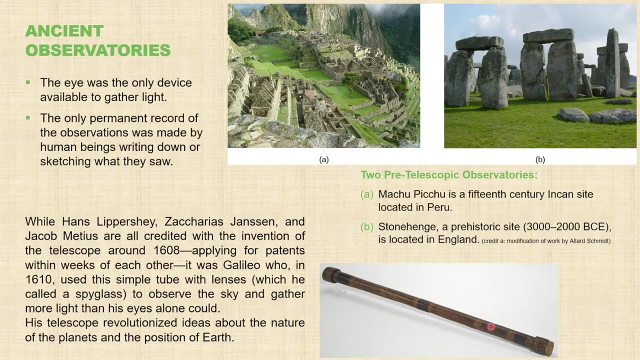 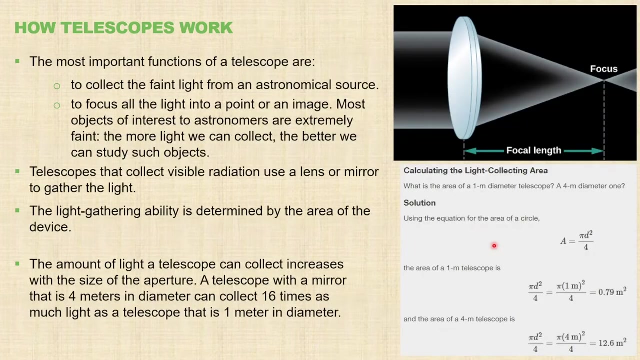 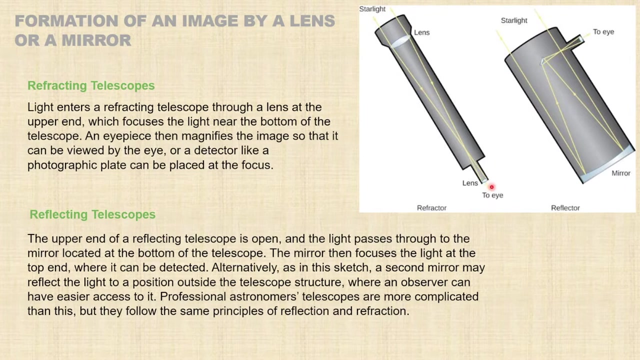 But if we don't stop, it magnified by another lens, and that's an example of simple refractor telescope. here Light rays entered from one end, it converged to a focus where the image is formed, and now that image can be further magnified by another magnifying lens, convex lens. This type of telescope is. 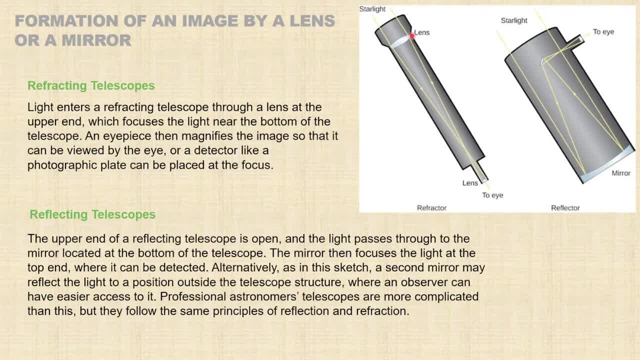 called refractor telescope. It refracts lenses, refract the light, because lenses are. you know they. they're not opaque, They transmit light. The other type of telescope is the reflector, like this one: here is a concave mirror. This is polished on the backside so it reflects light, so it's. 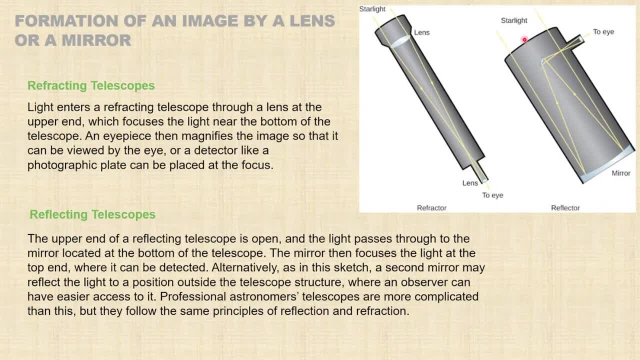 that's why it's called a reflector telescope. It has a very wide opening in this edge here, like the Hubble. the Hubble Space Telescope has a very wide opening and bigger that opening, more light can be collected. So the mirror. 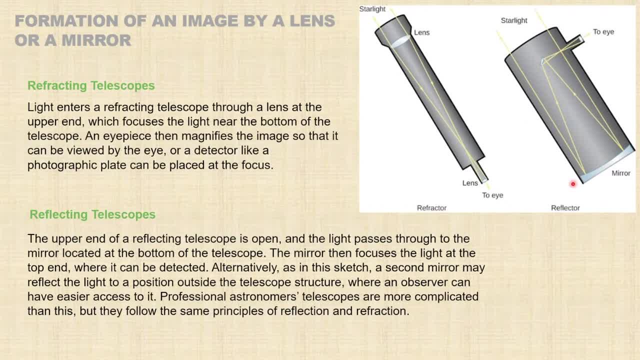 surface area of the mirror is you have to draw. that can be a little bit. smaller mirror has to be bigger. bigger area, more light And all the starlight that hit the mirror here gets reflected And based on this curvature here right, this curvature here has certain focal. 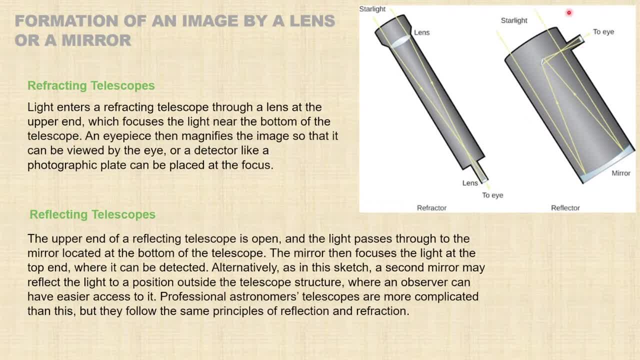 point, meaning all the parallel rays that come from a distant source. when they hit this curvature or the concave mirror, they reflect back to a point, they converge back to a point or at its focus, And that's where the image is formed. And to view it a little, another little trick: 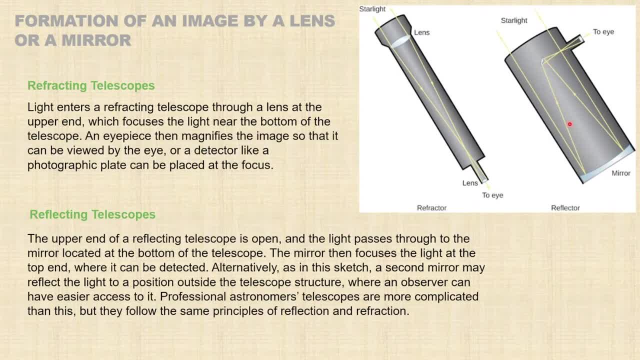 place another small mirror here, because now all this light rays is converging to a smaller area. Put a small area mirror there which reflects back towards another opening And there we can put a magnifying glass and we can observe that distance, distant object Could be a star, could be planets. 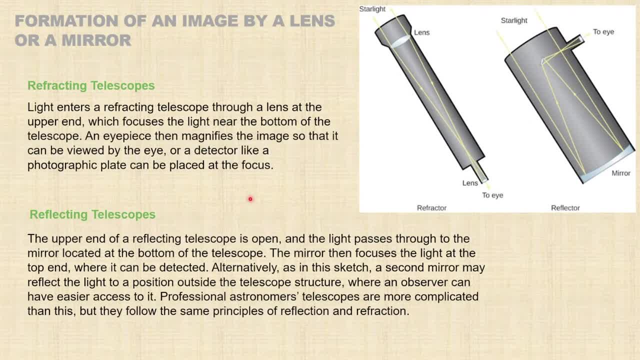 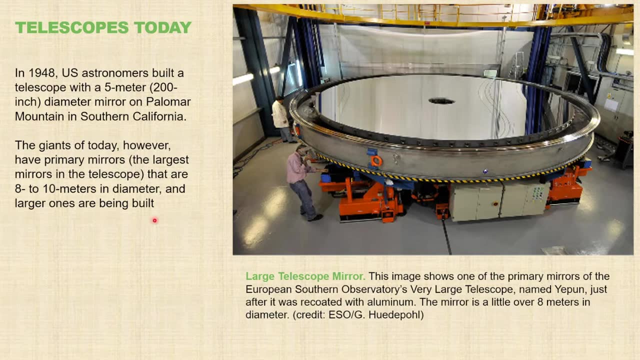 or even galaxy. We do see. we can see our nearest galaxy to the Milky Way, Andromeda, using such a telescope. Okay, Going from a very simple like half an inch diameter telescope, you know, within a hundred years, 200 years time, in 1948, US astronomers built telescope. 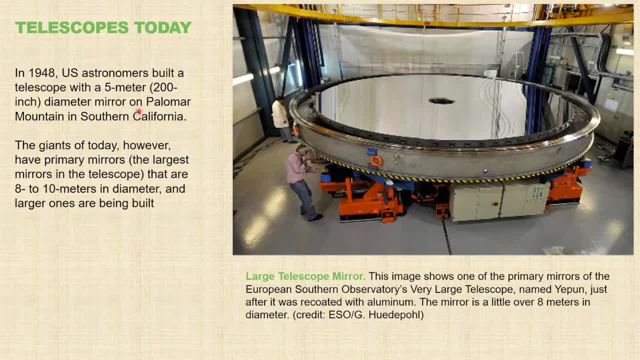 with five meter diameter, going from one or two inches to 200 inches long telescope, And that's the Polymer Mountain in Southern California. That's, this is not the Polymer 1.. This one is different, The. this is the VLA, Very large telescope built by ESO, European Southern Observatory. 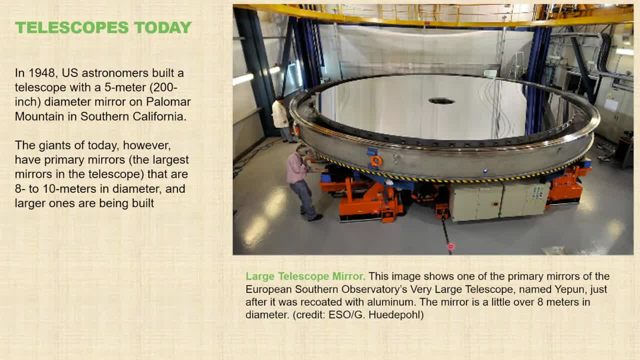 This is situated in Chile, Chile Mountains, and- And this one has the diameter of 8 meters, So very large collecting area- is a concave mirror. Light falls in that 8 meter diameter mirror and they converge to a point, producing some of the best images we have seen of planets in the solar system, the galaxies, the star. 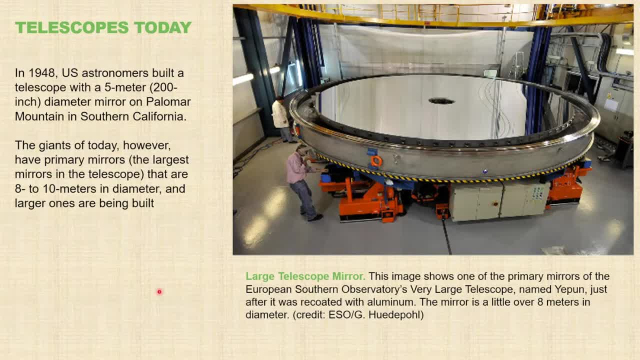 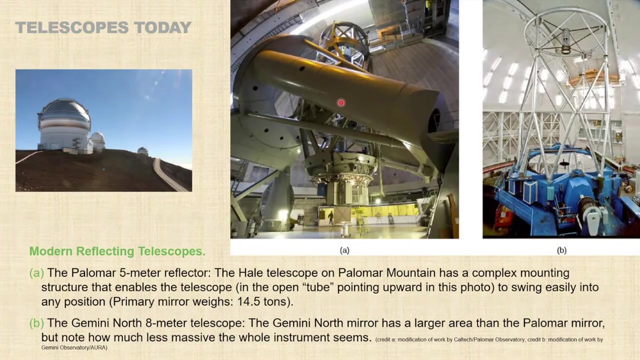 clusters, the stars, nebulas and whatnot. And that's 8 meters, there are 10 meters, there's 50 meters, that's being proposed. So it's only getting bigger and better. This one is the palomar in Southern California. here and there is a challenge. you know when. 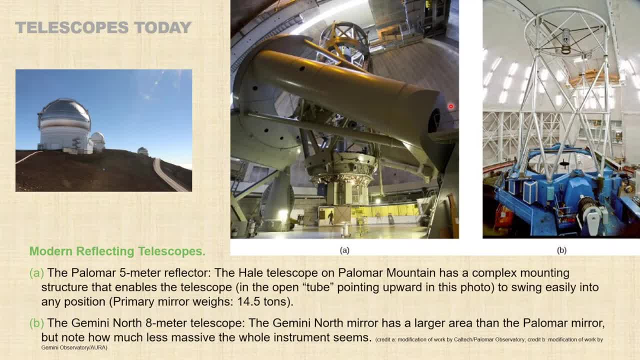 you. This is a big, bigger mirror. you know, back then with the technology, you know it got very heavier too. This one was 14.5 tons for a 5 meter telescope And when it's that big, you know it can shock due to gravity, due to its weight and distort. 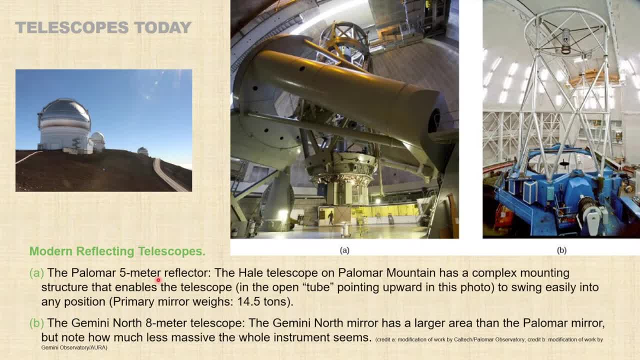 And so they had to build another 100 ton supporting system here. This was in 48. But later, after 50 years or so you know there are better materials were found, a better technology, where thinner mirrors could be built like this one: Gemini North. 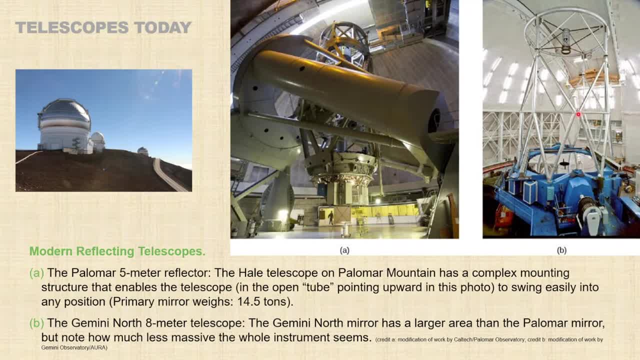 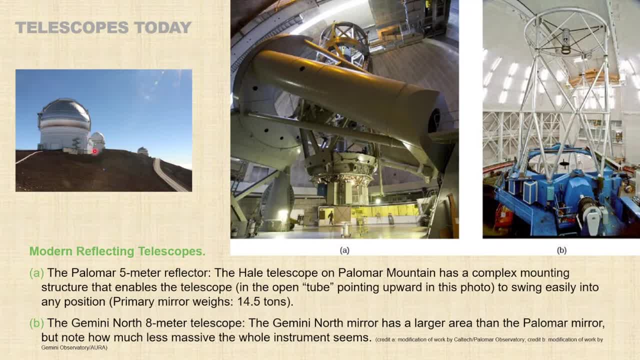 So I was at Gemini North here in 2007.. You know 6, Game 17,, no 16 December, And I had the opportunity to tour around the Gemini North. This is in Mauna Kea Mountains in the Big Island of Hawaii. 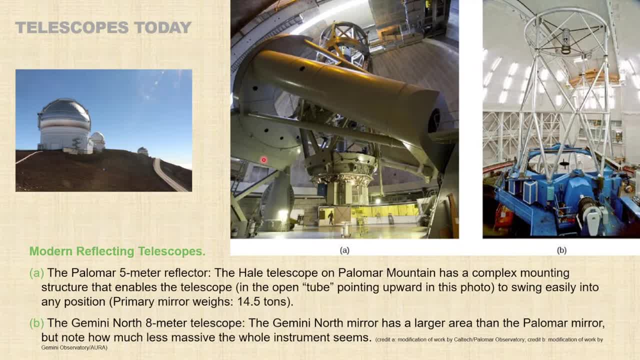 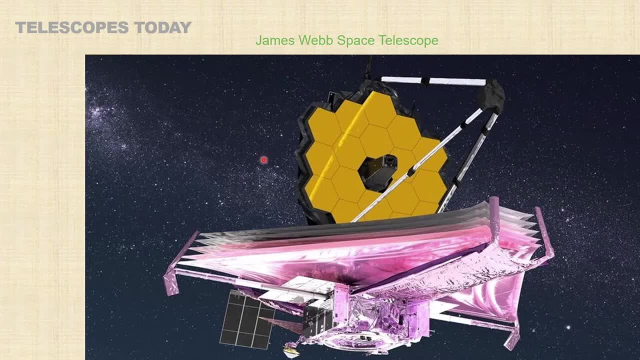 So you see, the top telescopes are getting bigger and bigger means better in terms of telescope. because of the size, it can collect more light. it can collect more faint light and it can collect light coming from much farther galaxies. right, we're talking about millions, billion light years away. 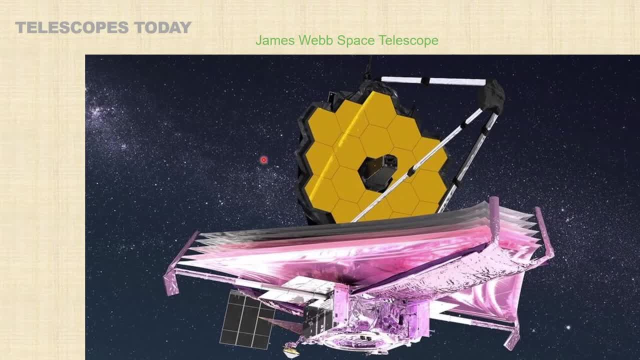 and this is what this, this telescope, is designed: the james wave space telescope, the most expensive telescope ever built, more than 10 billion dollars. it was launched few months ago. it is in the process of um calibrating its equipment. it has these huge hexagonal meters. 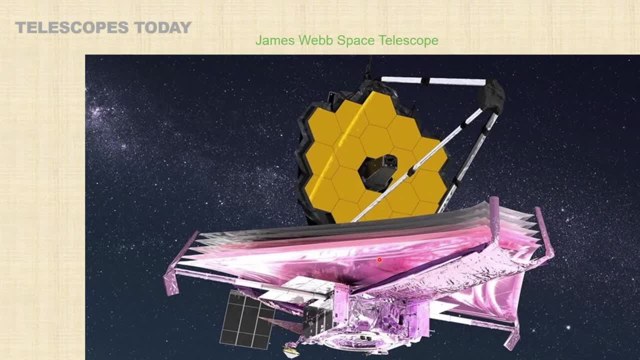 this are gold plated because you want mirror with best reflecting property. um, you know, the mirrors that we have reflect about 95, 96 percent uh rest is observed, so the information is lost. so whenever light is very faint- and we're not faint because we are signed by very bright uh led lights, but when 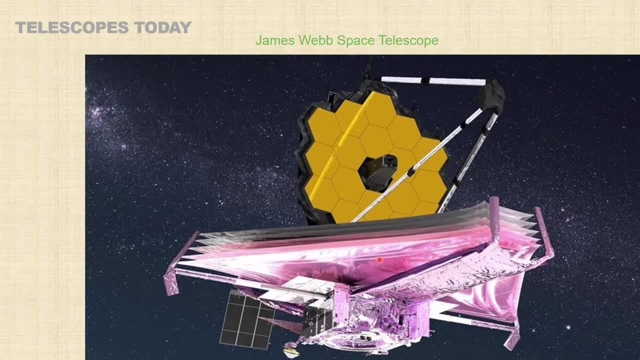 this thing is in space and you're trying to collect light that has been traveling for last 12 billion years. that's faint, so you want to collect more of that fed light in a larger area, and that's what this thing is designed for. you want- very you don't want any of that faint light to be observed by the 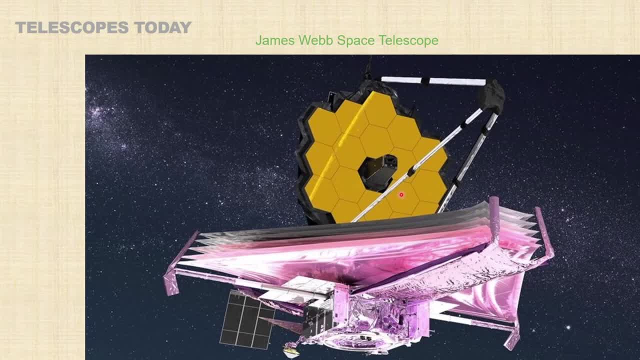 mirror. so you want all of it- 99.99 of it- to be reflected back to the detector here. okay, and- and this is the most technologically advanced telescope that we have- uh, you may have seen his first picture during the alignment process and i think they it'll go into full commission, uh, starting july or? 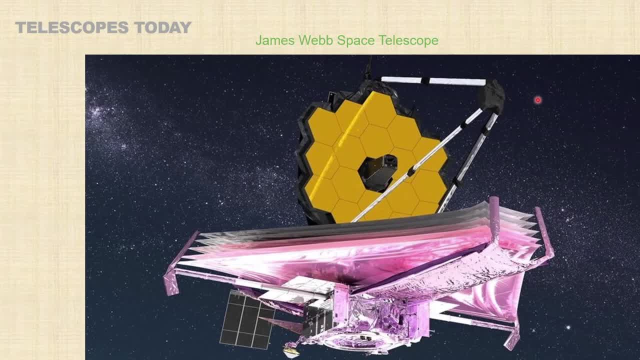 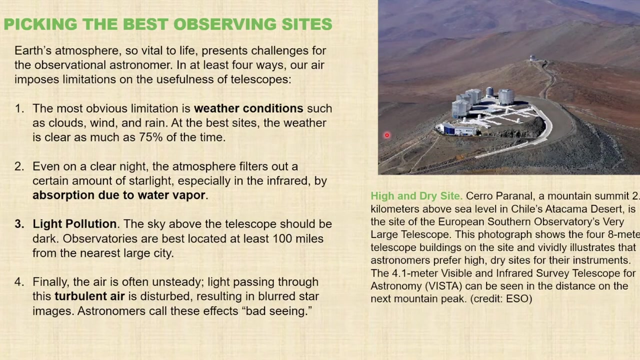 show and again. the goal is to find or to detect the light from the earliest stars that are far less away from us: the land-based telescope. we have certain challenges for using this telescope and one is the weather. okay, especially if we are doing optical. in the visible range we should be able to see the light should be able to pass through the. 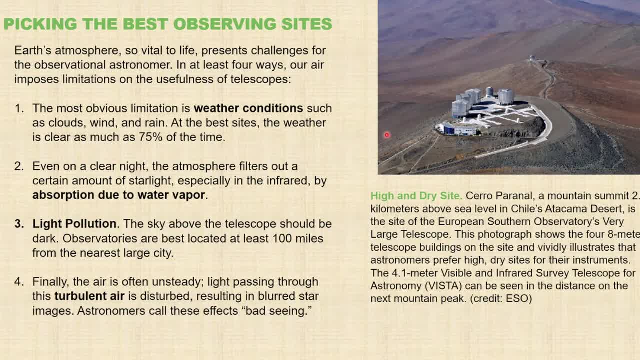 atmosphere and hit the telescope. but if it's rain, wind, cloud, and so that's the challenge, we have to overcome that, and so the best place on earth to put built telescope is where it rains less. so the weather is, you know, fairly constant. it can be hot, because this one here is the desert in chile. 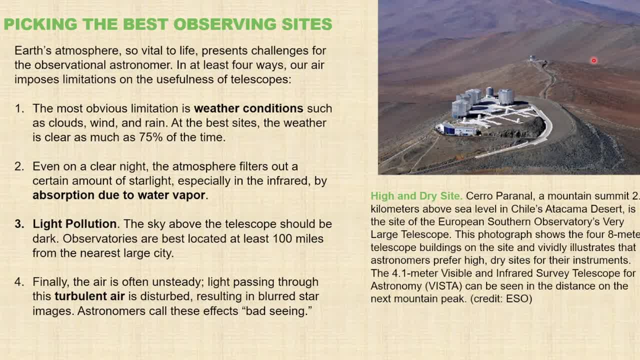 atacama desert: um. i don't think it has rained there in the recorded history. no clouds, it's at much higher place. very dry, dry weather is good if it is moisture, it has atmosphere. it has moisture in the atmosphere, the water vapors. those water vapors can absorb. 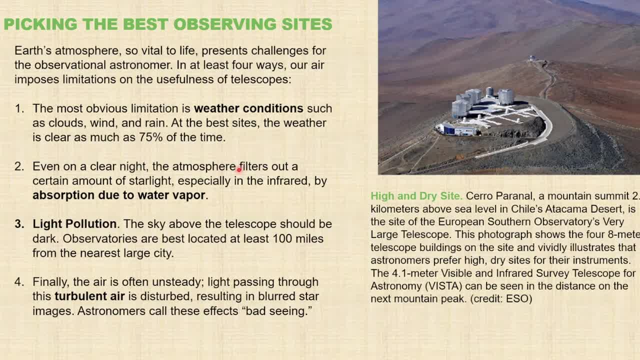 the light coming in and emit it on infrared radiation, and that distorts the image that you're trying to take. so, dry is better and, of course, it has to be much, much farther away from the city, as a matter of fact, to have a good night sky, visible night sky. 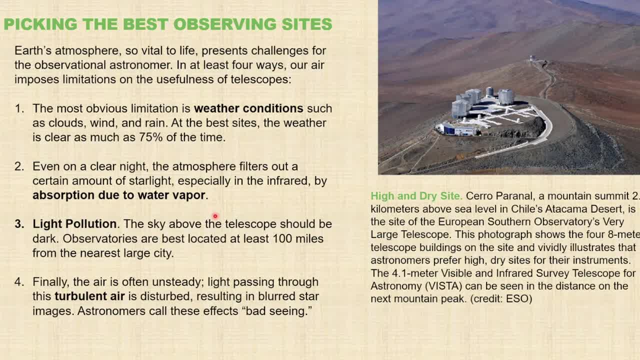 if you really want to enjoy the night sky, you have to travel as far as 100 miles from the city. okay, so that's why this, this telescope, like our biggest best in texas is what's the? the west texas observatory, mcdonald observatory in west texas by the guadalupe mountains. that's like 400 miles from here. 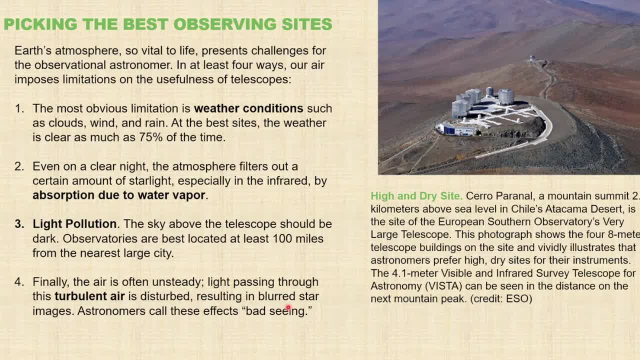 uh, we do have one observatory and that mcdonald observatory played a critical role in finding, detecting planets, exoplanets that orbit two stars, a tattooing like planet called gamma cpi. we'll look into that planet and observatory when we do exoplanets. and finally, the turbulent. 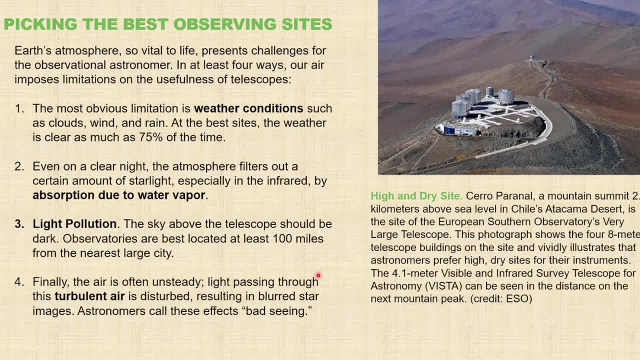 because the air is moving fast, um there, you know, there can be turbulence, uh, um, in the, the atmosphere, the molecules of the air, and that distorts the image as well and resulting in the blurry images of the stars or galaxies. astronomers call this term a bad scene. 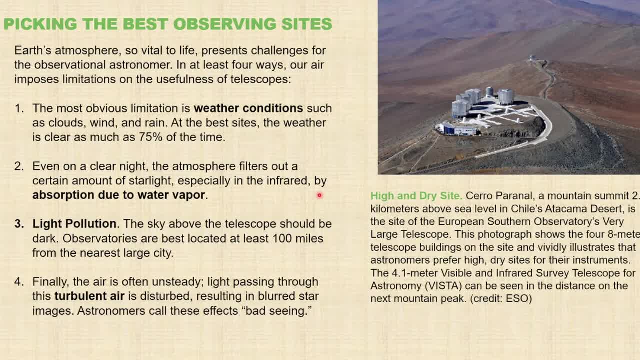 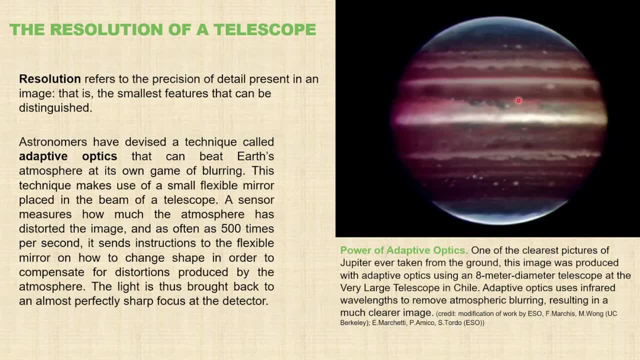 however, there's a way to uh, to get around this turbulent air. this is the uh highest resolution, clearest image of a jupiter taken from the earth's surface, earth's surface nowadays. again, we can get rid of that turbulent air by something called adaptive, adaptive optics. 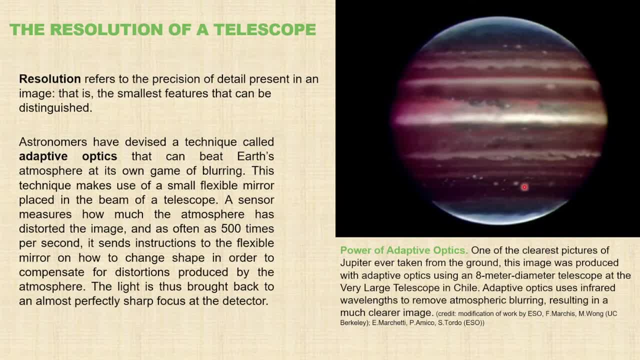 um, it's like ai, artificial intelligence. you know, computers are connected, sensors are connected within the telescope meter, where those telescope meter can be twisted and turned in a way to compensate for whatever the turbulence is. if turbulence changes, if turbulence causes the- uh, this image to distort by some degree, then we can adjust that mirror. the computer detects that. 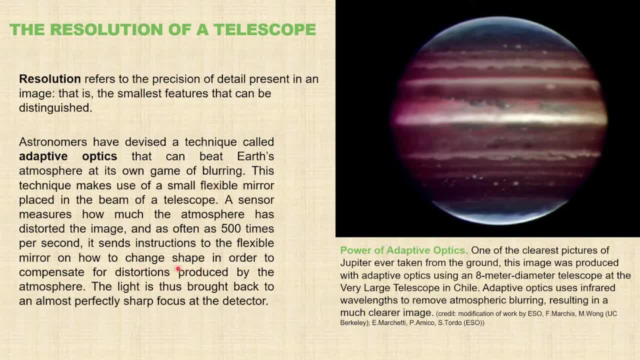 and computer automatically adjust those mirrors uh to compensate for the distortion and hence produce a sharp uh image uh in the detector. and that that that field or that technology is called adaptive optics, meaning adaptive optics: the optics adapts itself to compensate for any external error. and again, resolution refers to the precision of details present in an image high resolution. 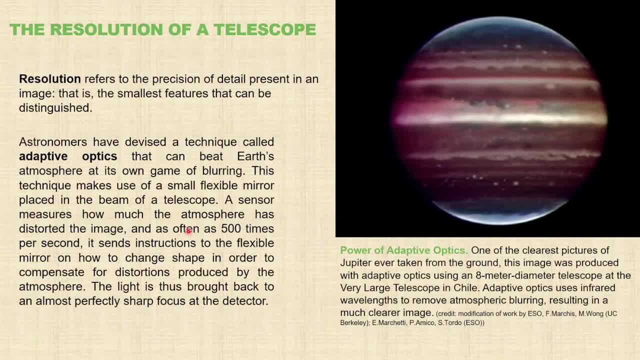 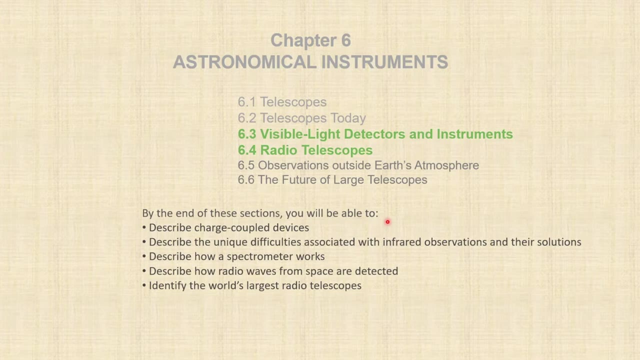 you can expand it more, you can zoom in more and you can see more details of its structure, uh, in the jupiter or other other planets, or even moon? now let's look at the detectors itself. what's there in the detector and other type of telescope like radio telescopes? 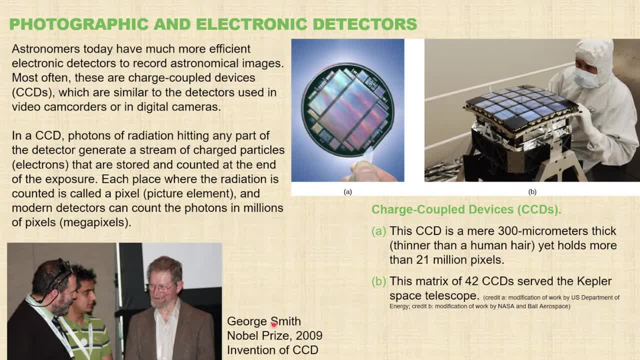 in, uh, in 1990. uh, this person here, whom i had the honor to meet with in 2010 in portland, oregon- uh, his name is george smith. um, he was working in bell labs in new jersey, i believe, and he found a way to store the. 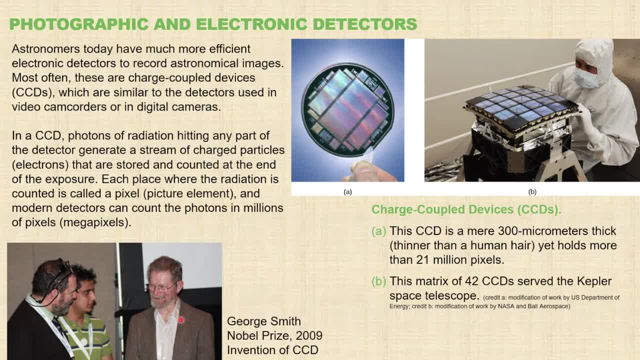 energy excited by the photons and that energy which is carried by the electrons. okay, let me rephrase that: he invented something called ccds, charged couple devices. and how that works is whenever a photon, a light particle, a radiation particle, whenever photon hits a surface, that surface, or a detector, a metal, 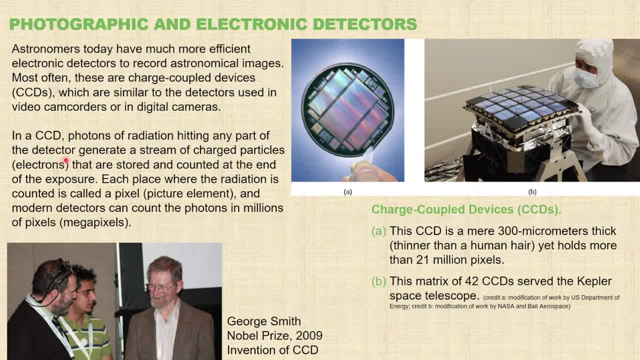 that surface has electrons, that photon energy, whatever energy the photons come with. again, photon is the light particle. so right now your body is emitting out photons. that's why i can see you, those, those light particles, the photons, are entering through my eyes and it's hitting the receptor inside my eyes, in the retina. 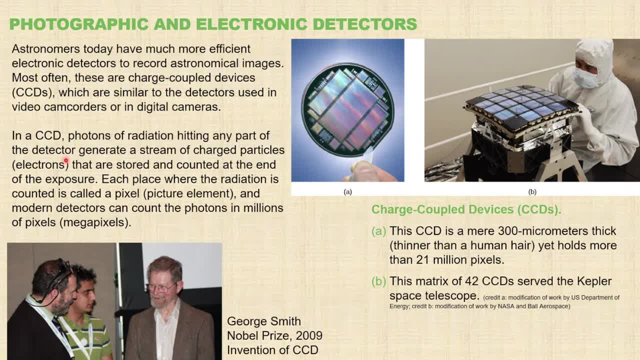 and that excites the electrons, that those electrons charges move to the brain and my brain interprets that energy and makes me able to see. in the same way, the photon that hits the plate excites the electrons and that excitation energy is carried by the electron and is stored somewhere in the detector. 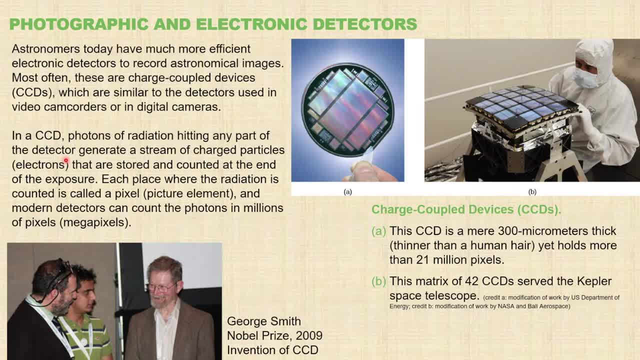 and when it collects all the different photon energy, it's able to store basically a picture of that object. and this cct revolutionized everything. remember the tape camera that you had a film, you had to have a film in it. and when light light enters those light. 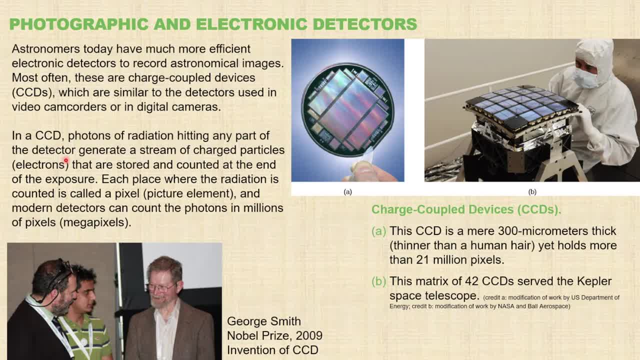 it has sensors, photographic sensors in it, chemicals in it. that's one technology. but with ccds we didn't didn't need a film anymore. That's when we started to get all these digital cameras. Our phones have it. This is everything has CCDs, And so for that contribution he was awarded Nobel Prize in. 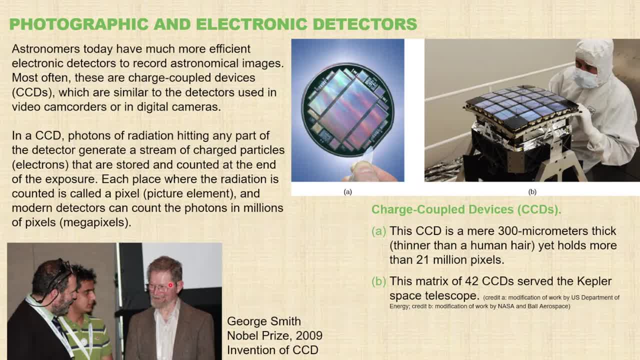 Physics in 2009,. George Smith, And that's what we use in the telescope. The telescope, the mirrors lenses. they collect light, that they form images, but those are directed somewhere. They have to be detected and stored for later use Right, and we use CCDs like this one here. They have grown. 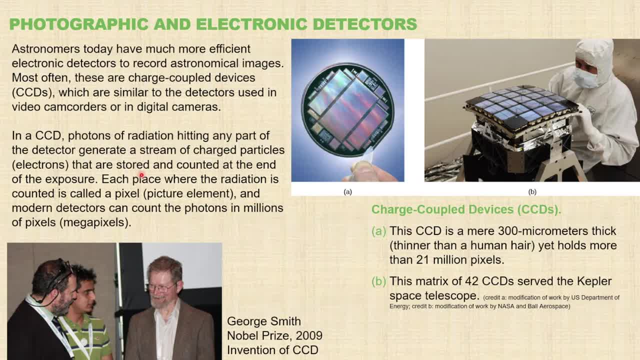 of course, the efficiency has increased of those CCDs And, as a matter of fact, it's a place where the radiation is counted: One, four, five, six, seven, eight, nine, 10,, 11,, 12,, 13,, 14,, 15,, 16,, 17,. 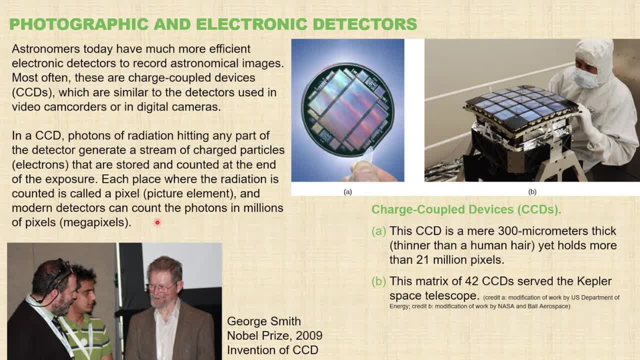 18,, 19, now, 10,, 20,, 21,, 22,, 23,, 24,, 25,, 26,, 27,, 28,, 30,, 32,, 33,, 34,, 35,, 37,, 38,, 39,, 40,, 41,, 42,, 44,, 45,, 41,, 42,, 43,, 44,, 44,, 45,, 46,, 5,, 52,, 44,, 45,, 46,, 57,, 57,, 49,, 52,, 43,, 43,, 45,, 47,, 50,, 53,, 46,, 57,, 58,, 51,, 52,, 54,, 47,, 58,, 51, 52.. 51, 52,, 52,, 57,, 58,, 54,, 59,, 52,, 56,, 59,, 50,, 57,, 56,, 57, 56, 58,, 55,, 55,, 58,, 56,, 59,, 57,, 59,, 59,, 60,, 60. 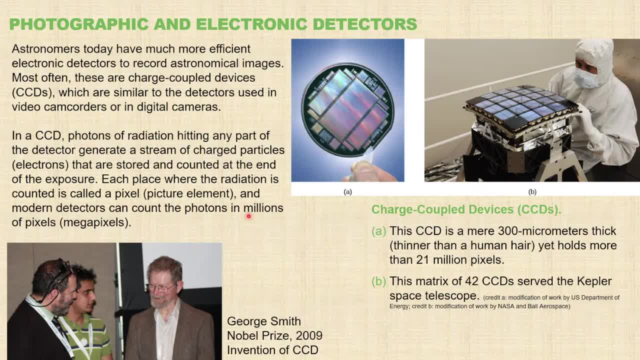 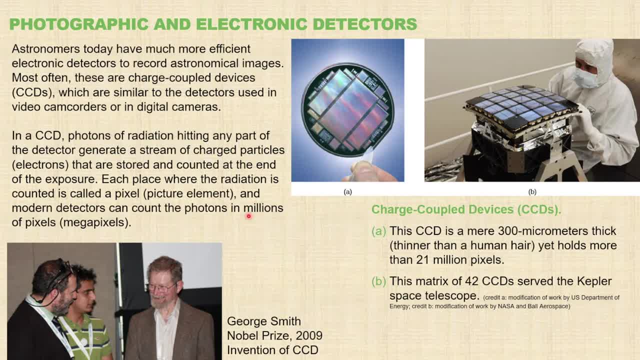 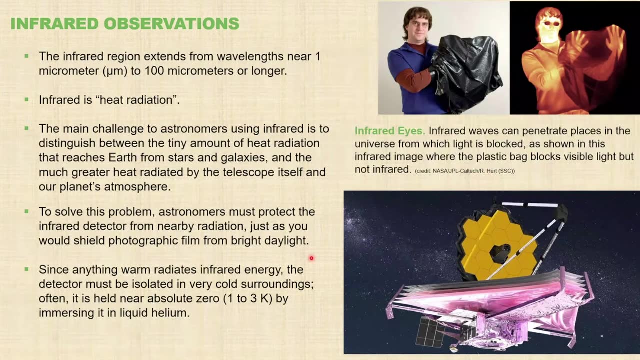 And more is. the pixel is like the grid: more grids, More resolution, higher resolution. There are also infrared observations. Hot objects emit infrared radiation, not just hot. even any vibrating charges can produce infrared radiation. It's part of the whole spectrum- electromagnetic spectrum. 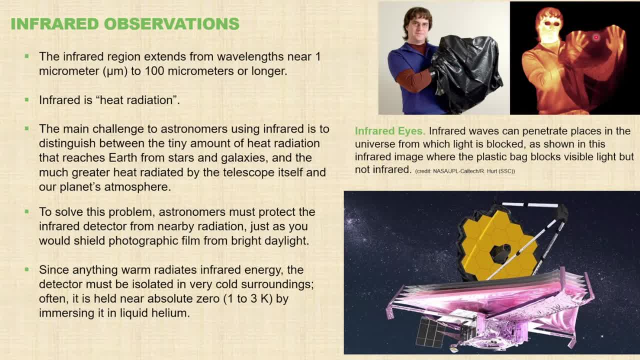 your normal body versus. it's covered in a thin plastic, but the plastic does not emit any heat or infrared radiation. But if it's looked through a camera that can detect infrared, a person who would glow and seem like this- even the radiation coming out of the hand- and are detected. 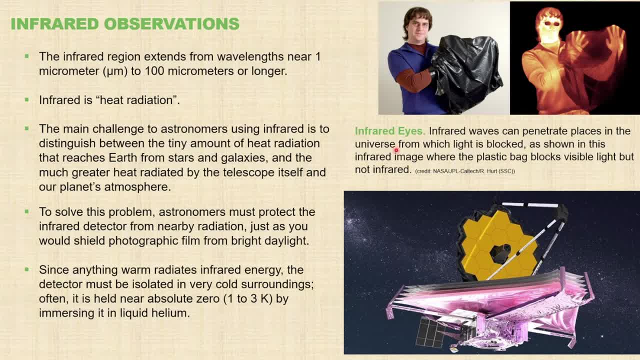 And again, infrared is a is a heat radiation. The one challenge with building infrared telescope is that, since it detects the radiation from hotter object, the telescope itself has so many electronics It's constantly creating some form of heat So that heat can be detected within the lens. 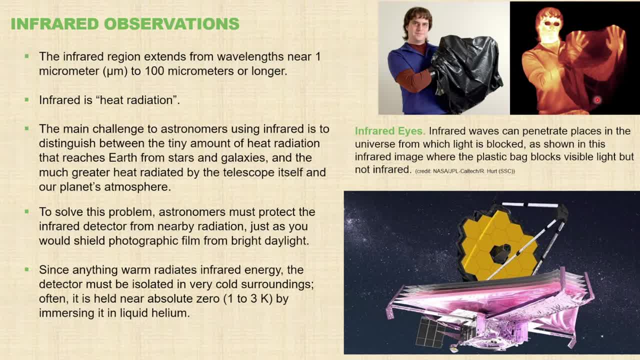 And can obscure the image Or the actual radiation that you want- infrared, infrared radiation that you want from distant light, distant stars- When you're trying to measure the infrared radiation from a light light source that is 10 billion light years away But before that light can be detected. 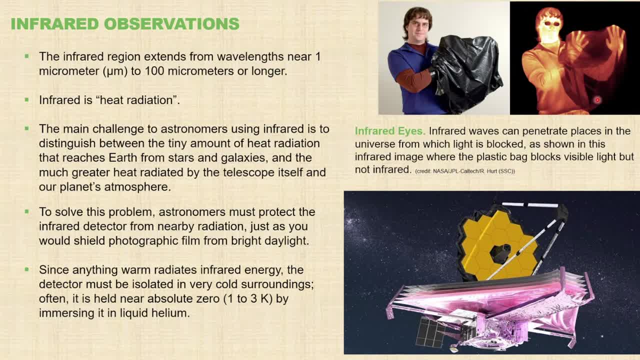 you have that background noise due to the heating. Is telescope Itself Okay and the solution is to that is there are two ways We can prevent that For the Earth based telescope: that these, this telescope, can be covered in a very cold surrounding, cold temperature. 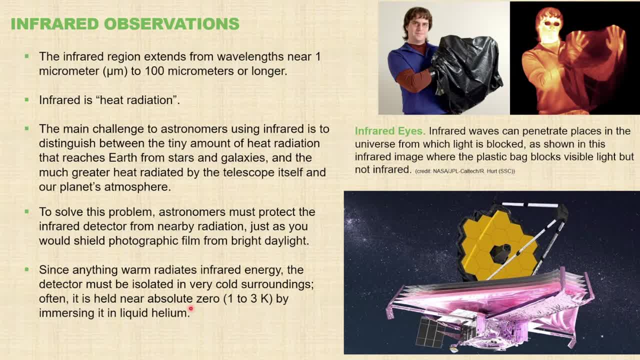 They can actually dip it inside helium or liquid helium Towards, you know, absolute zero temperature, So that radiates, that Radiates least amount of infrared radiation. That's like reducing the background, noise, the unwanted radiation, And only looking at what you want, which is the infrared radiation. 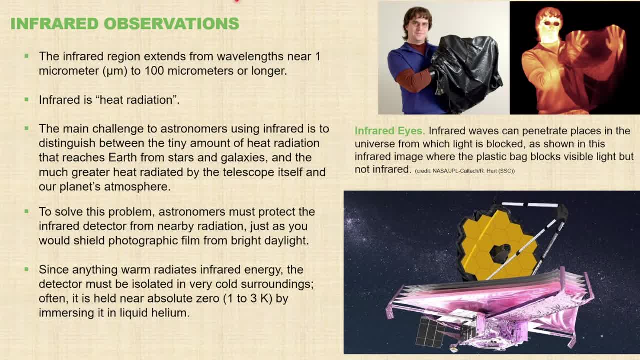 coming from a distant source. And the other way again, we can take telescope into space like James Webb Space Telescope. But even there we have a challenge because the Sun- in this space We're not getting too far from the Sun- is within the solar system. 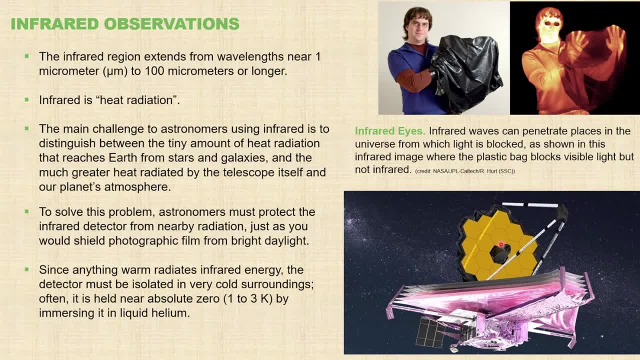 But the Sun rays, the radiation from the Sun can strike the, the telescope itself and cause that unwanted infrared radiation. So for that reason there are these Foils, these, these are almost football-sized field foils. Again, it always these. the telescope always faces away from the 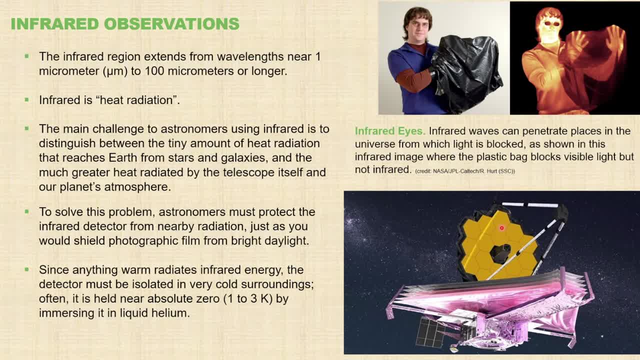 telescope and the foil blocks the radiation coming from the Sun and there are layers of foil Works like a insulation, So even some radius and interest through the first layer, the second layer stops it, Third layer stops it and there is no radiation passing through it and 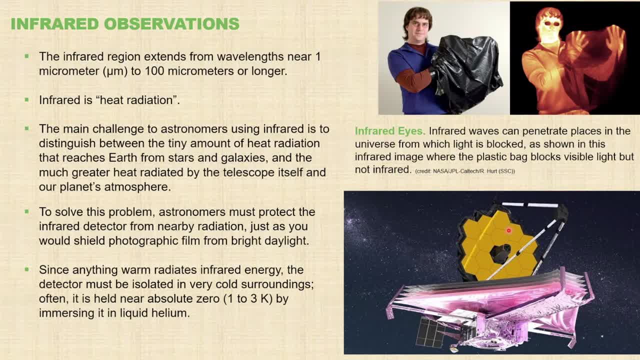 out in his space in one of the Lagrange Point In his space it that far It's very cold And so cold whatever radiation is blocked. So it's the best place for telescope like this one to observe any infrared radiation coming from the light source from. 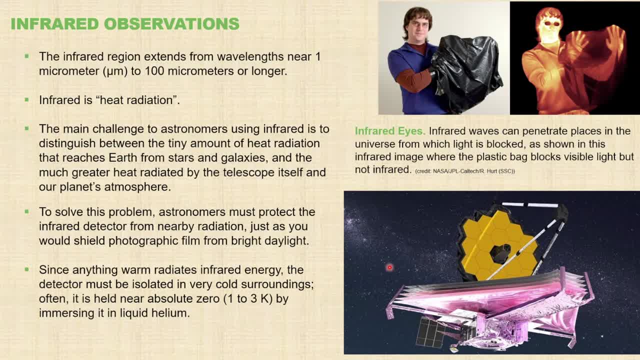 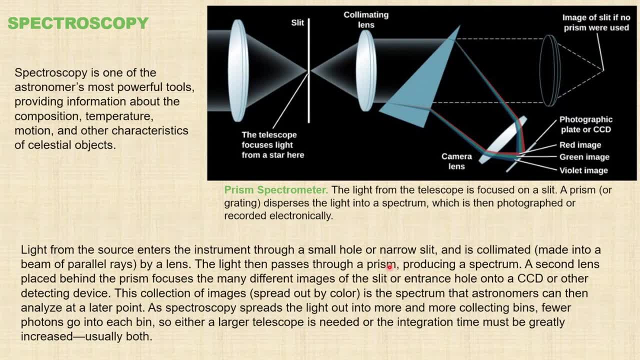 Like says, the stars that are 1012 billion light years away. That's the whole visible universe. And the spectroscopy. It's a device, you know, that converts a light ray into different spectrum of light. For example, light source is collected here by a lens. 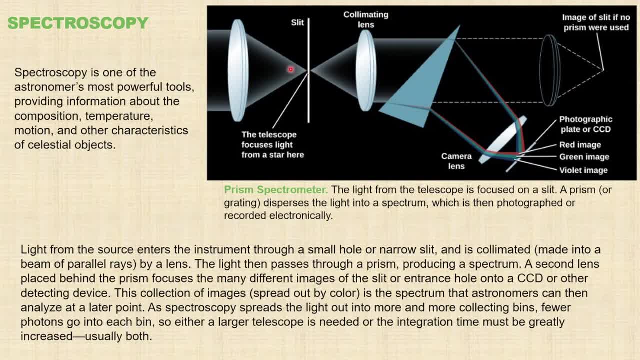 It's converted and sent to a small slit And it converges here, goes through a slit. of course this after that focal point it diverges again. but we have a lens, collimating lens, that sends these light source coming from the image here into parallel. 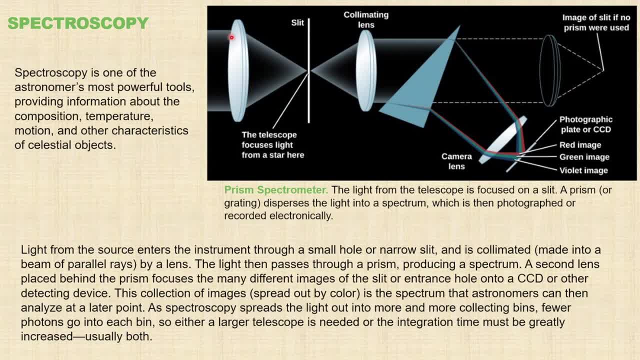 light rays or this is just opposite here To this lens: when and the light come in parallel and interest of convex lens, they converse to a focal point, but the source- light source coming from the focal point, when it hits the converging lens they immerse. 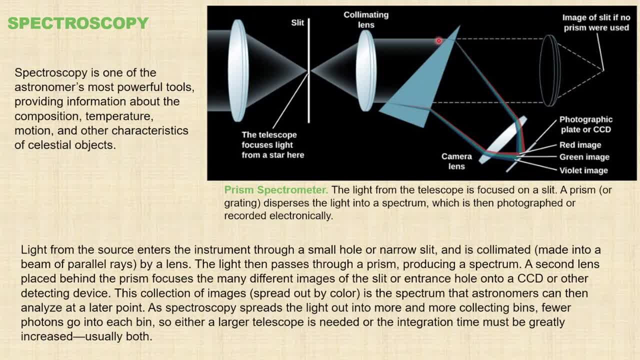 parallel opposite. So now this parallel light rays are passed through a prism And light rays get refracted here because the light rays have different These. this light ray consists of multiple, multiple wavelength light, because visible light extends from red to violet. Depending on the energy of the photons, they refract differently. 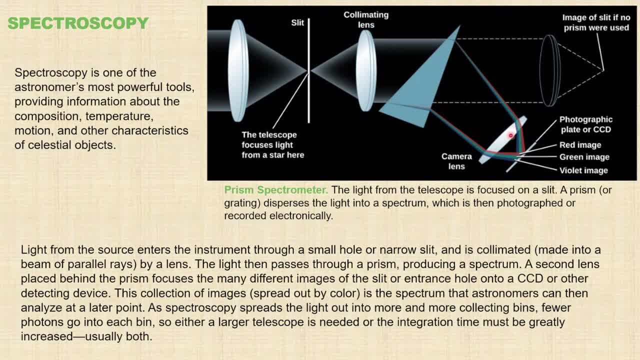 The bend differently and so certain. so basically, we are separating lights with different wavelengths and they are sent to a different detectors. if you want to measure something In the red, you put your detector in the in the red image, red detector here, which forms a red image versus green, versus violet and so on. 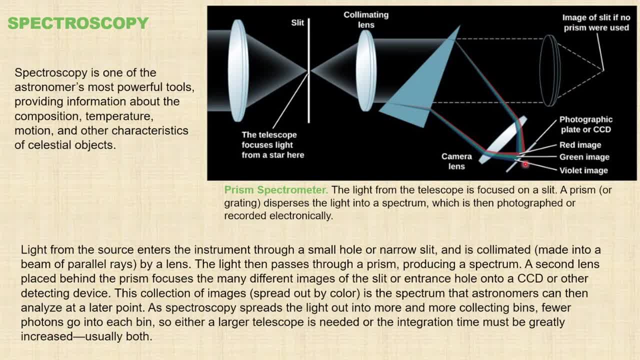 So here are multiple detectors that have CCDs or photographic plates, And that's the spectroscopy. And one challenge is that because the light source is spreading out, the photon count gets decreased. this light source, Now we are breaking into multiple colors And so same amount is now being detected by multiple detectors, but it's 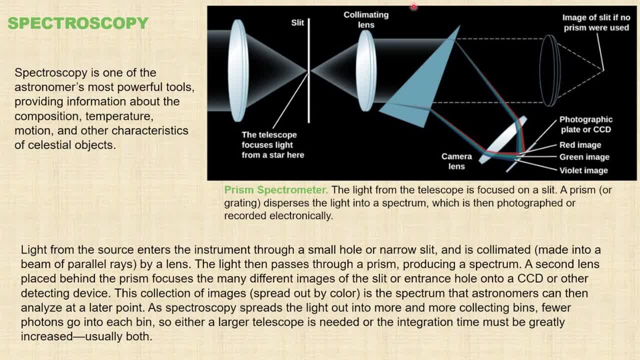 detector has very less amount of photons compared to this- all photons here, That Interesting collimating lens. So for that purpose we may need to increase the size of the lens- More area, more light- or increase the exposure time, The detection time. 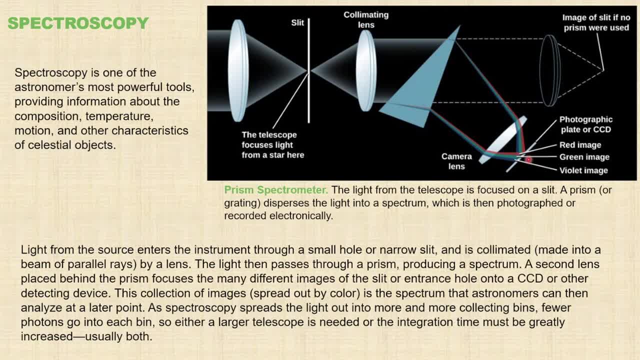 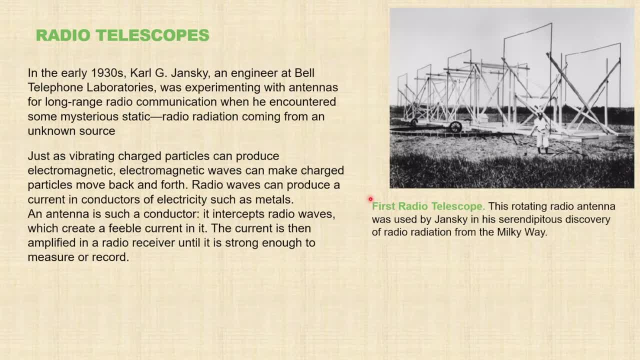 Or the time that we collect the photons. We may have to increase that significantly, or both. The radio telescope. So in our electromagnetic spectrum This is the radio range: Very large wavelength, longer wavelength, Small frequency and as it moves towards the gamma rays and x-rays, past visible. 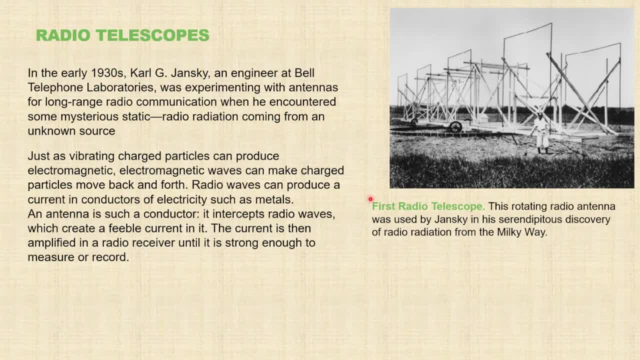 Light. This is our visible Section And this is our infrared section. here This is gamma rays and x-rays. So We can build telescope to measure each section of this spectrum, to detect light or photons Of each wavelengths. Optical means visible. 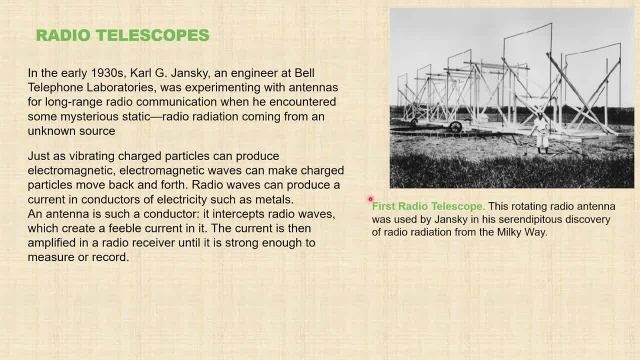 Okay, Infrared, And now, accidentally, A radio telescope was built. Antennas, Same like your radio antenna, your TV antenna, You have a car antenna above in your car. These antennas, they detect these radio waves coming from your FM station. 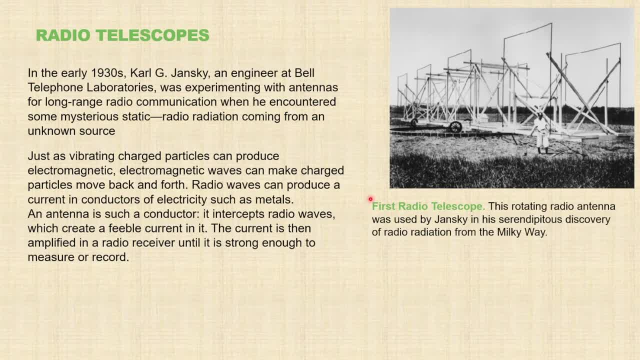 And these waves carry energy. These radio waves Transfer that energy to the electrons that are in your antenna and those electrons Carry that energy to the machine in your radio. call that decoder, because it's decoding The sound wave, The voices, the songs, the music that was converted into radio waves. 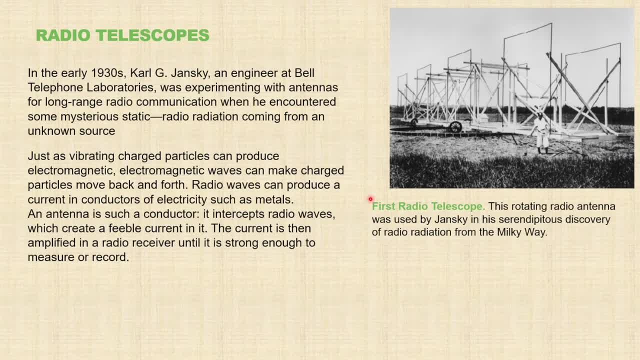 Your antenna receives the radio waves. That excites the electrons in the antenna. Now that electron, which is electrical, which carries electrical waves, electrical energy has to come. that has to be converted into sound waves. So you have a decoder And that sound waves is sent to a speaker. 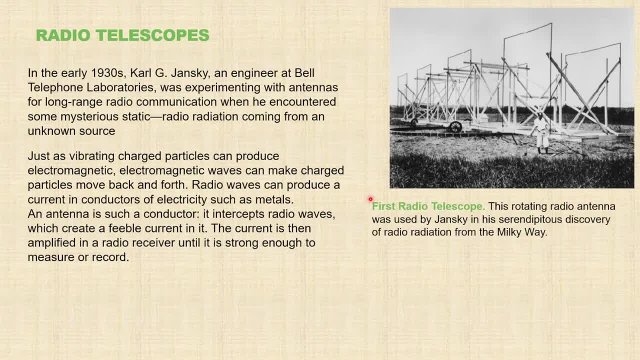 And you hear the voice. So there is a quarter and decoder. first It has to be coded Sound waves has to be coded into electromagnetic waves. Electromagnetic waves are decoded into sound waves And during that process, this guy, this guy, 1930 Jansky, was receiving these radio signals not being generated by anyone on the earth. 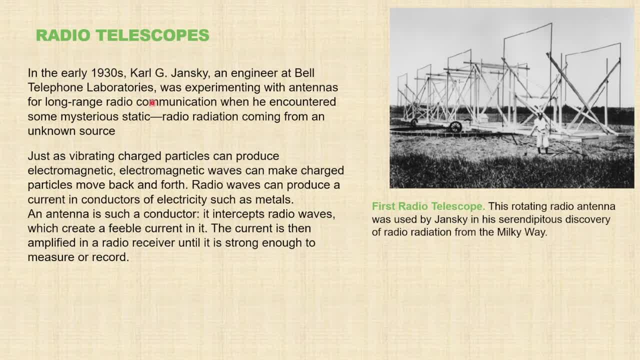 As a matter of fact, later he found these, These radio waves coming from Other objects In the sky, from other stars, because the lighting is stars, stars, The supernova, explosions and there are other events that produce these radio waves Hundreds of light years away and they travel everywhere in the universe. 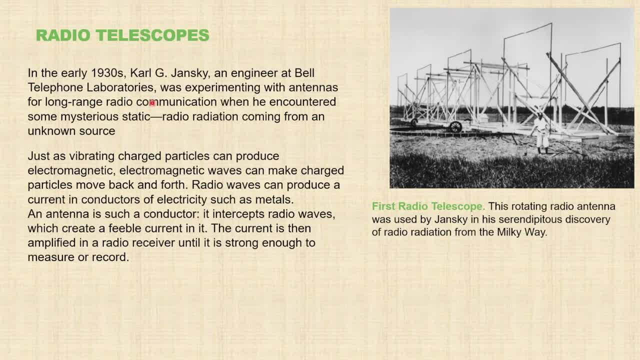 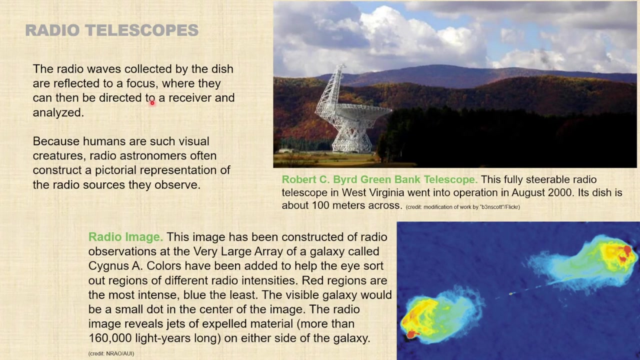 Some of them happen to hit His devices and he was getting that static Radio signal all the time and hence a rebirth of radio telescope Happened in 1930.. Later on, scientists more formalized it, make it more precise, Just like the visible light. 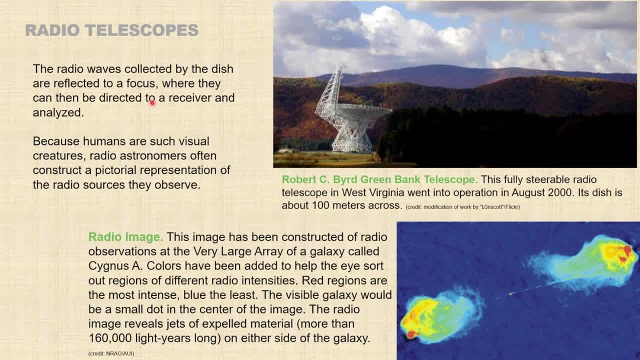 When light ray enters A concave mirror, it reflects back, Or a mirror you can see yourself, because the mirror reflects light that's a visible light. These, these telescope, Radio telescope, x-ray, gamma rays, behave the same way. any of these, any wave in this spectrum here gets reflected, like this curvature here of this. 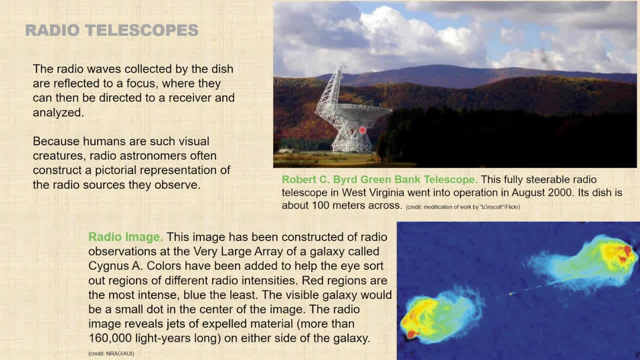 This antenna here. the radio waves coming in hit This curvature space and they reflect back to a focal point all the light. the radio waves hit this curvature here and they reflect back to a detector here on the top And that signal is sent to your electronics, to the CCD, and 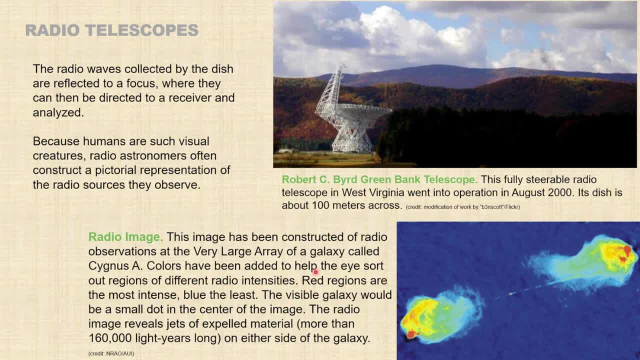 Pictures like this can be created. this is of the galaxy called Cygnus a, The radio signal coming out of the galaxy, And, of course, the colors are added, because the radio, we don't see it, but, based on different energy, we can add artificial colors to it. for example, in this case, red regions are the most intense. 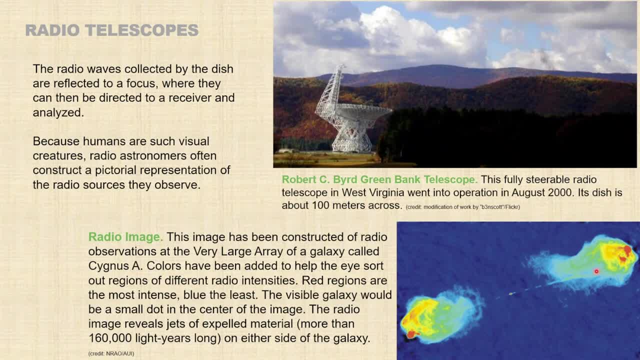 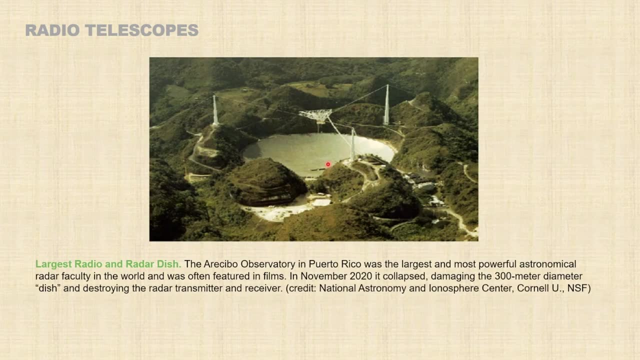 And the blue, the list, And this is a hundred sixty thousand light years long, This distance here. And you have seen other popular radio telescope like the Puerto Rico, which collapsed, I think two years ago, Is no longer operational. this use, the same technique, this disc here, the radio waves coming in. it's the disc and all these radio waves are reflected. 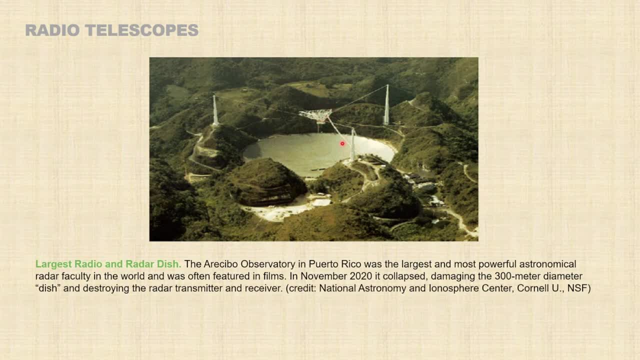 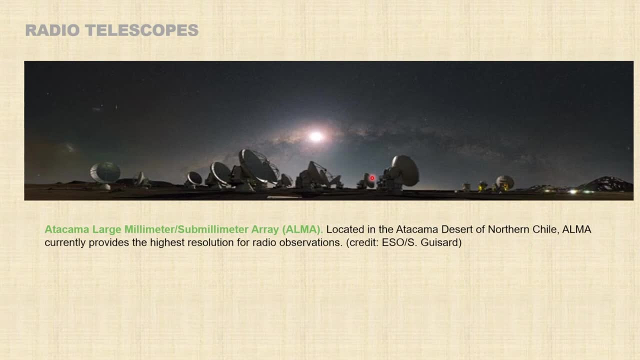 Back into a detector Here on the top and that signal is taken out for processing. This is a good example of radio telescope. there are many other. this one is at a camera in Chile, Northern Chile, These all this here. they all detect radio waves coming out from, not just from, solar system. 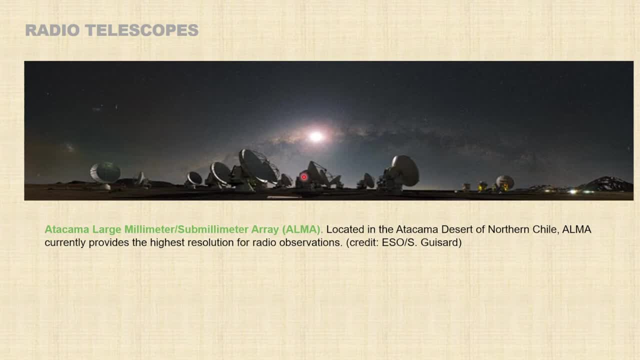 The, the interaction between our our nearest, Largest planet, Jupiter, and the moon. that interaction- the IO, IO, Jupiter's moon IO- and the Jupiter interaction create, creates this certain radio wave signal very peculiar, And that signal can be detected here on Earth. We can hear that static sound. 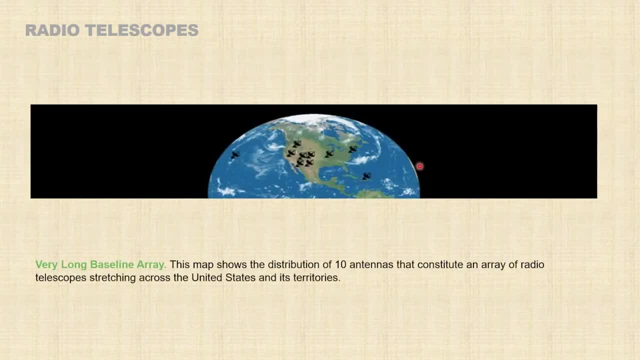 And not just from our planet, from distant galaxies as well, And we can form an array of Such telescope. because it only collects certain, It's limited, so if you had to collect more light, it's like increasing the surface area of a mirror. This is called very long baseline array, and some radio telescope are placed in Hawaii, in the Caribbean, from Maine to Southern California, to Northwest.